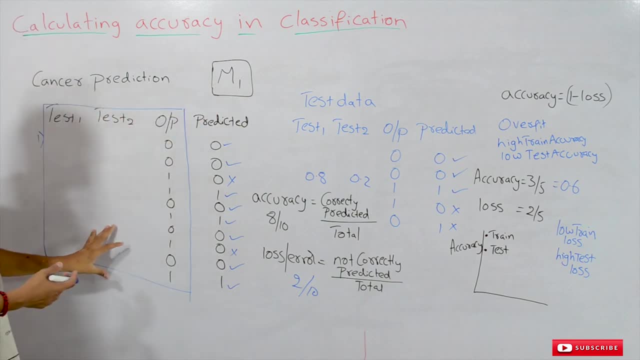 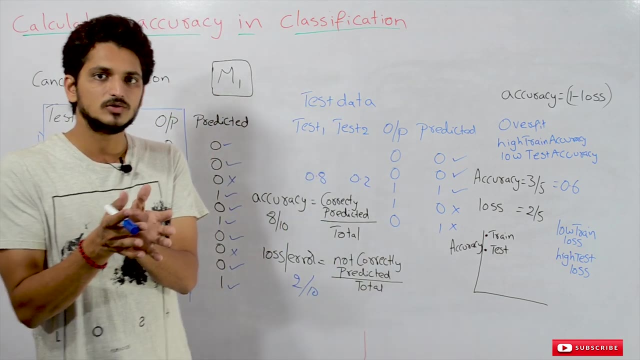 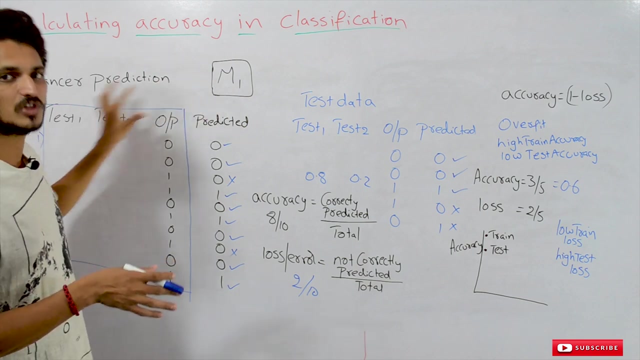 So the model will train based on this training data. So now we can use this model for predicting our future data points. So the predicted values of this training data set is like this: Based on this M1 model, the prediction values of this training data set is like this: 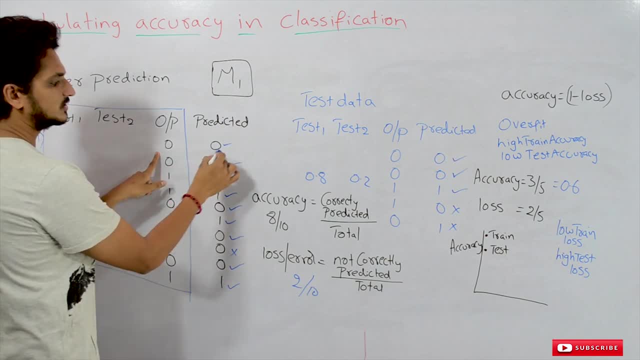 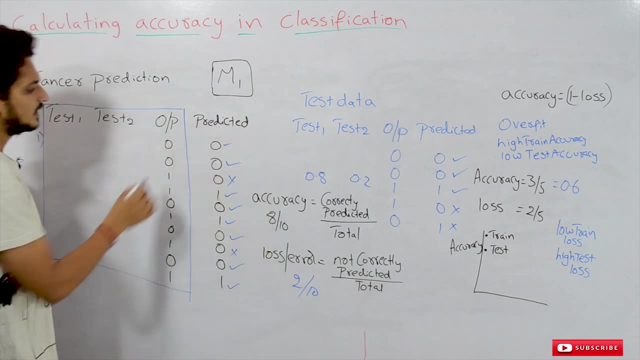 For the first data point, our predicted values is 0.. Second data point is 0.. Actual value is 0.. Predicted value is 0.. That's why it is correctly predicted: 00. correctly predicted: 10. not correctly predicted. 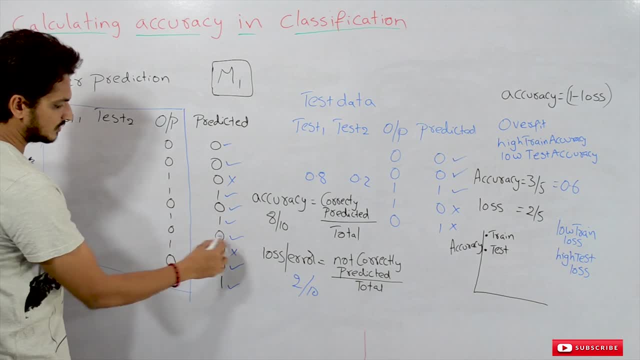 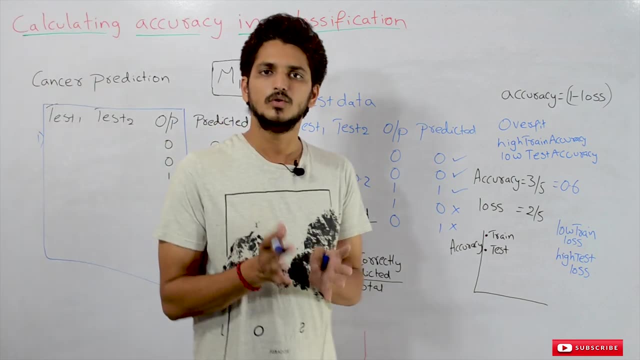 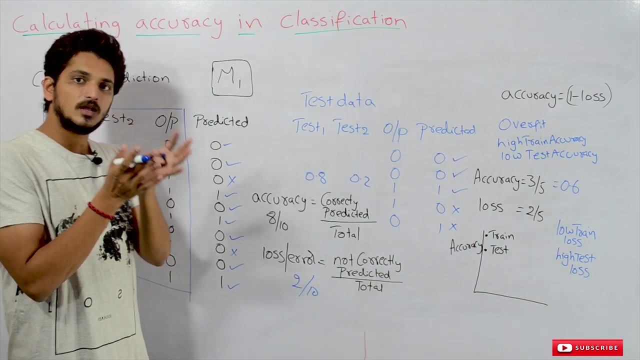 11- correctly predicted: 00, 11, 00,. 10- not correctly predicted: 00, 11.. So this is how we do in machine learning. Now, how to calculate the accuracy of this model: Number of data points that are correctly predicted on this training data. 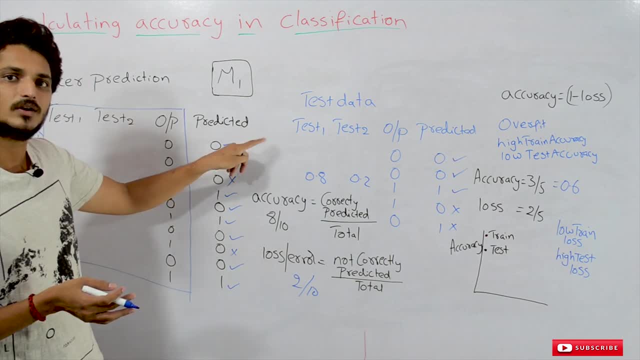 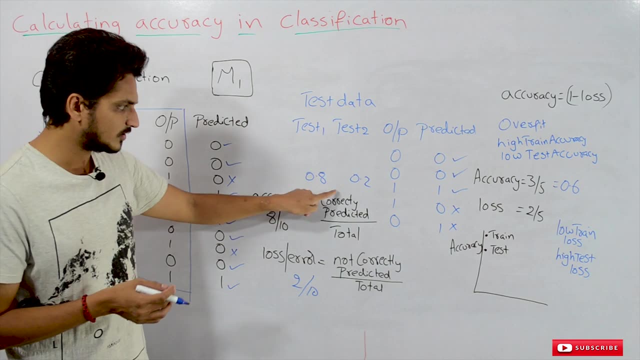 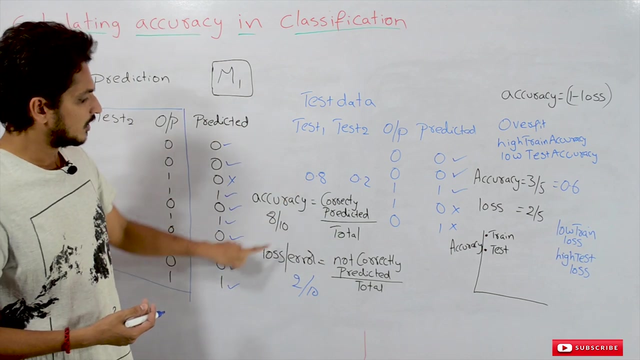 We call it as training accuracy. So out of 10 points, 8 points are correctly predicted. So that's why the accuracy is equal to correctly predicted values divided by total number of data points. 8 by 10, that is 0.8.. 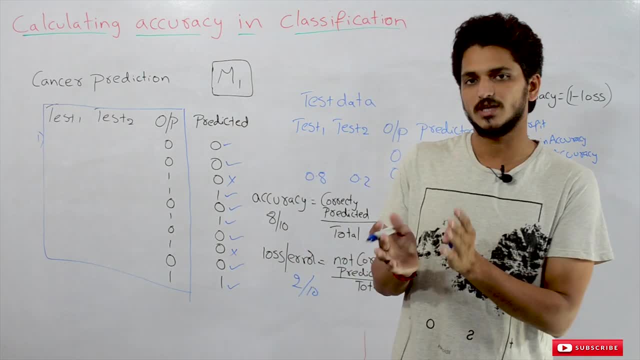 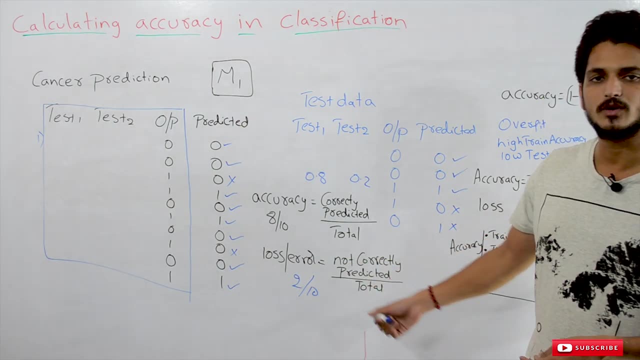 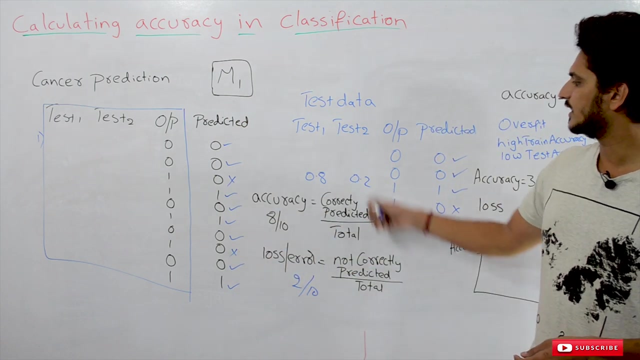 Loss value or erroneous value. We use these terms interchangeably. Loss is equal to number of not correctly predicted values divided by total, That is out of 10,. 2 values are not correctly predicted, So 0.2.. 2 divided by 10, that is 0.2. 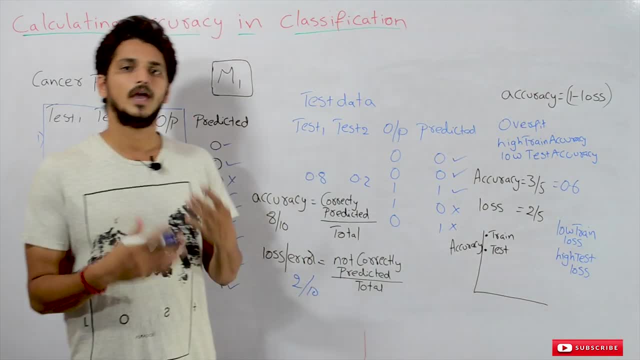 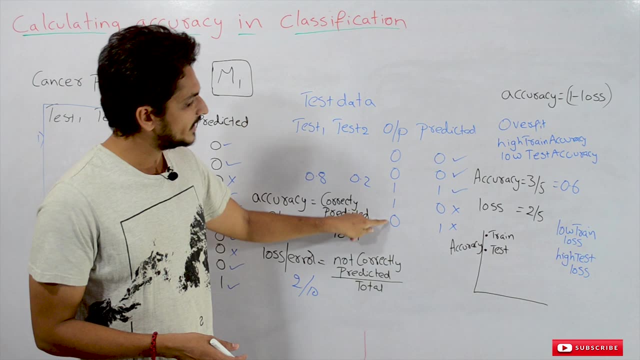 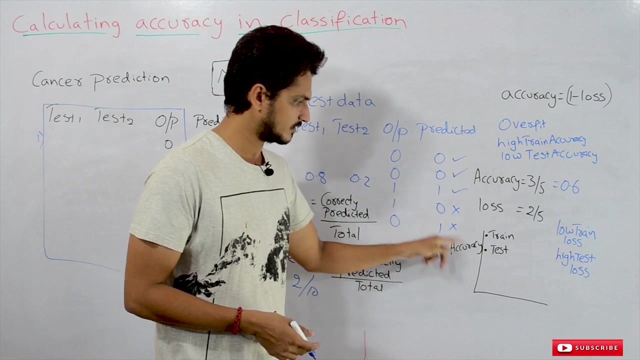 The same way we calculate the testing accuracy and testing loss. So out of how many values we are having in testing data, We are having 5 data points. Out of this, our model: predicted: 00 means correctly predicted, Correctly predicted, wrong, wrong. 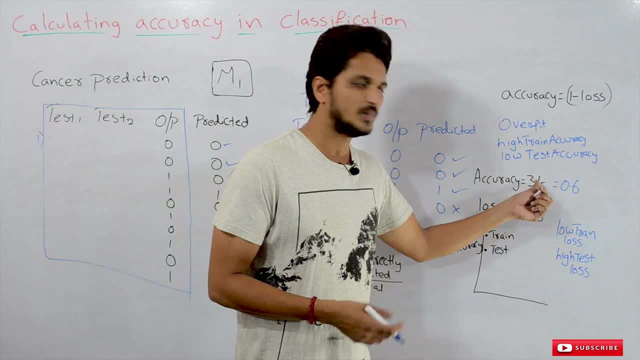 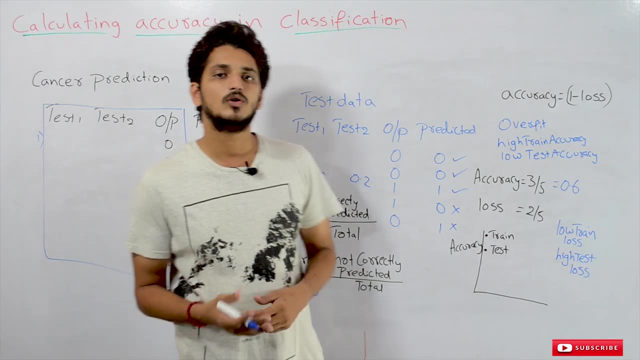 So, out of 5 data points, 3 of the points have been correctly predicted. So accuracy is equal to 3 divided by 5, that is equal to 0.6.. Loss is equal to 2 divided by 5. that is, 2 divided by 5 is equal to 0.4.. 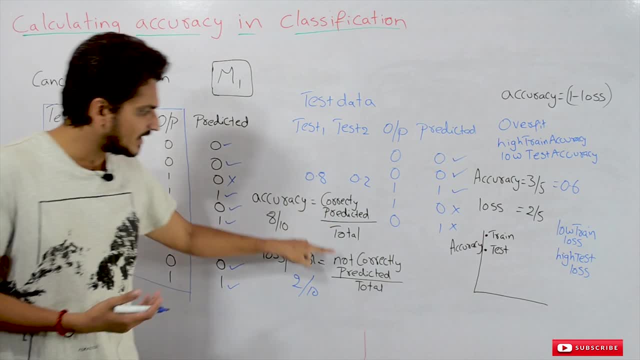 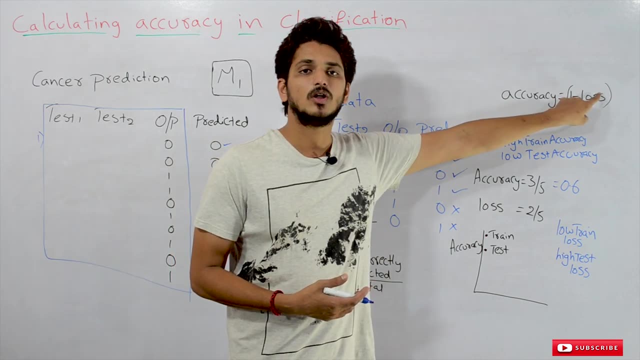 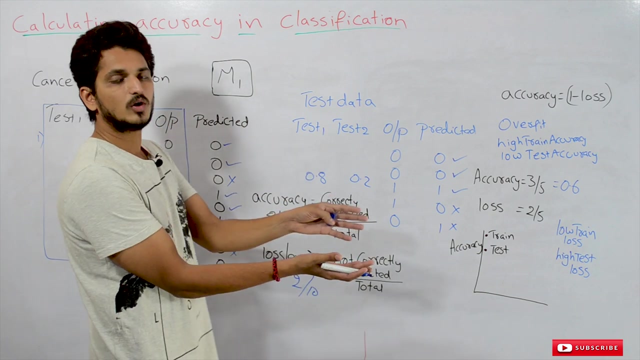 Here. what we are doing is we are just calculating the percentage of correctly predicted points. That's why accuracy is equal to 1 minus loss. Just we are calculating the probability. So accuracy plus loss is equal to 1.. Total points we will get: 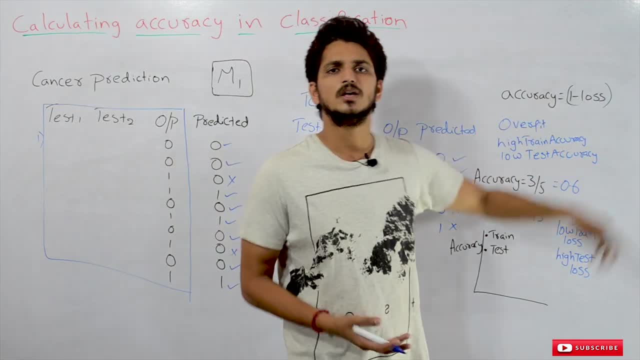 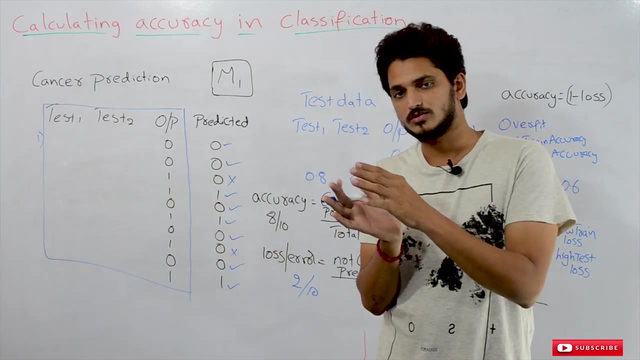 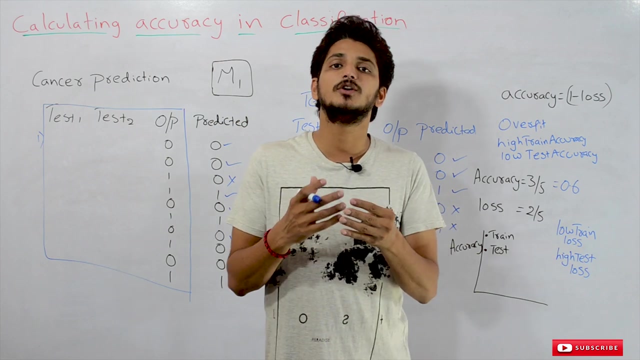 That's why accuracy is equal to 1 minus loss. So why we want to calculate these values. We will plot these accuracy values on a graph. We use that graph for finding how best our model fit to the data. This is what we will calculate, using these values. 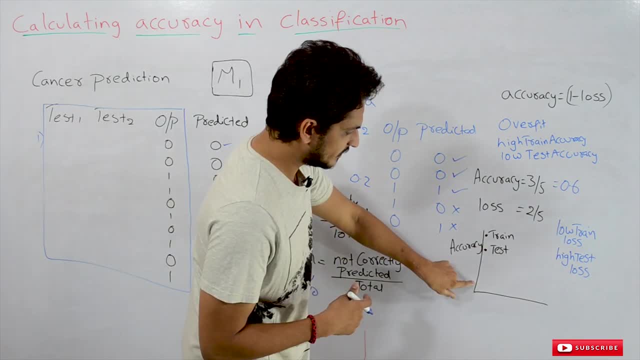 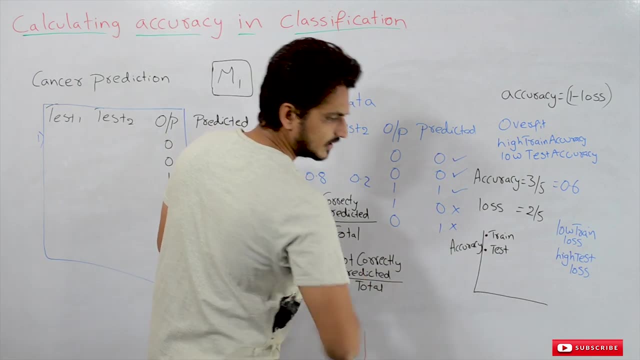 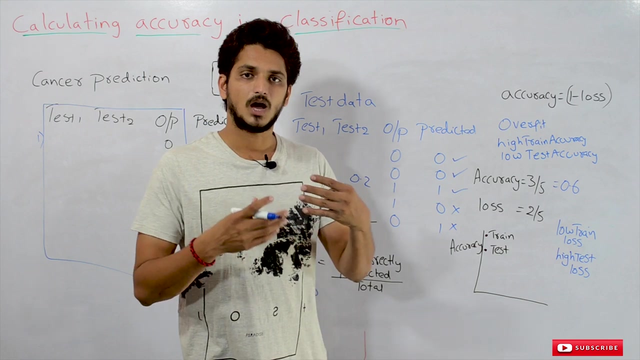 Let's say, on the y axis we are taking the accuracy values And we plotted the training accuracy And testing accuracy. The values has come like this. So why we use these values? We use these values for identifying how good our model fit to the data. 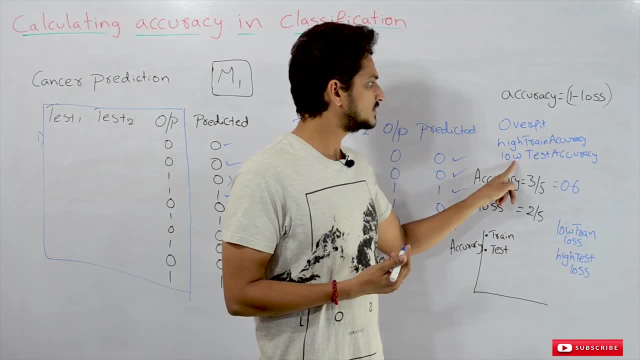 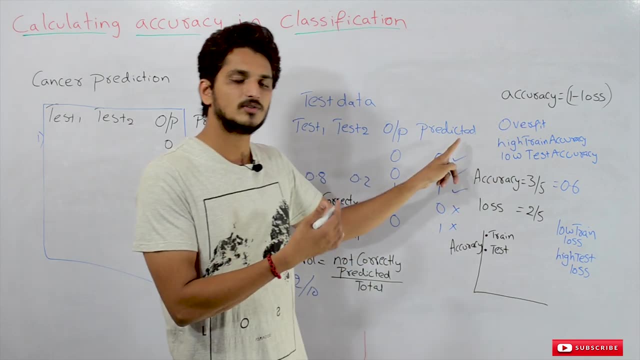 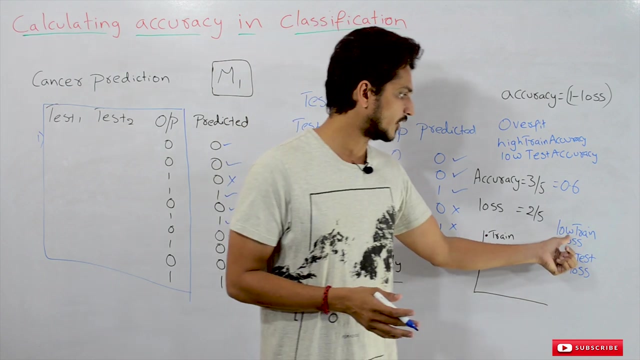 If the training accuracy is high and testing accuracy is low, then we call it as over fitted model. This we already discussed in our previous concept over fitting concept. Why we are showing it here is: some of them will plot loss points, Some of them will plot accuracy points. 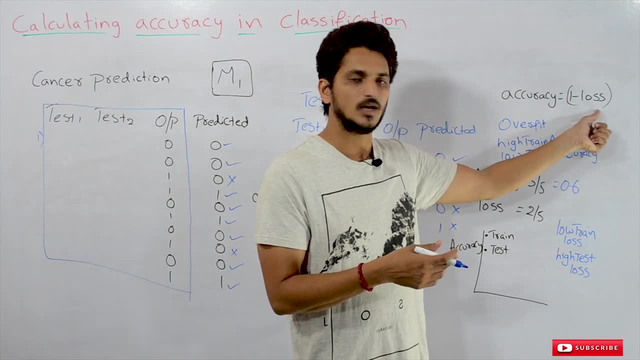 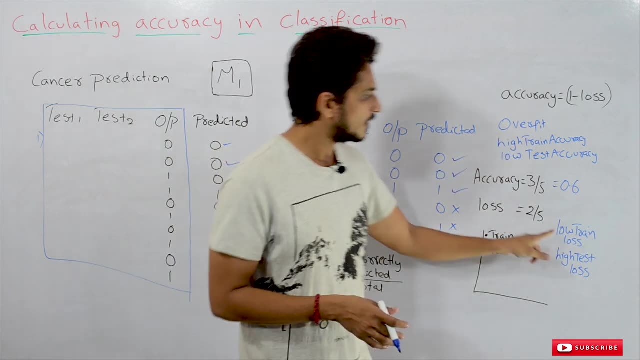 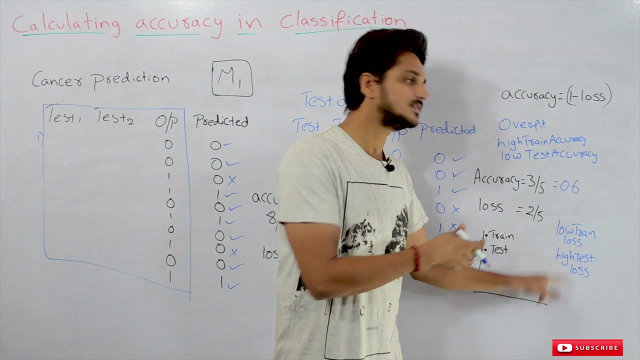 So which is accuracy is equal to 1 minus loss. You have to understand the difference. If the graph is given in loss, how we calculate the over fitting- Low training loss, high testing loss, Then we call it as over fitting. If the plot is accuracy over fitting. 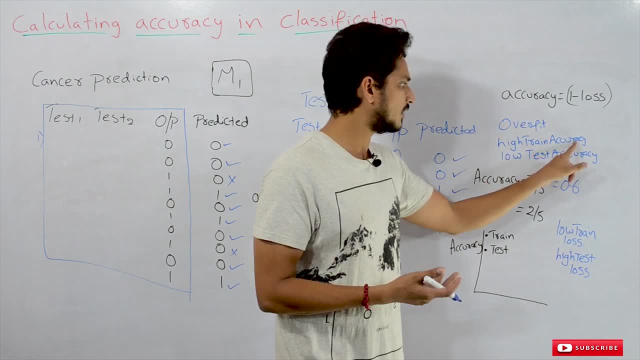 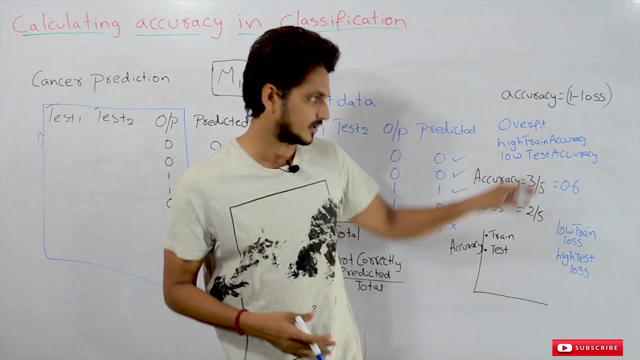 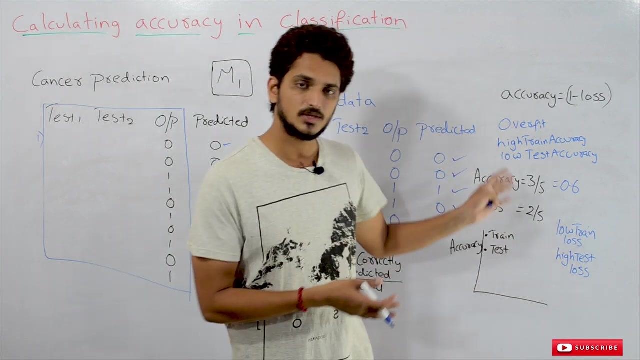 How to calculate over fitting, High training loss, Low testing accuracy. This is what This accuracy model we use in our models. That's why we are showing this here. Whenever we deal with the machine learning models, we will plot the accuracy plots and we will identify over fitting and under fitting. 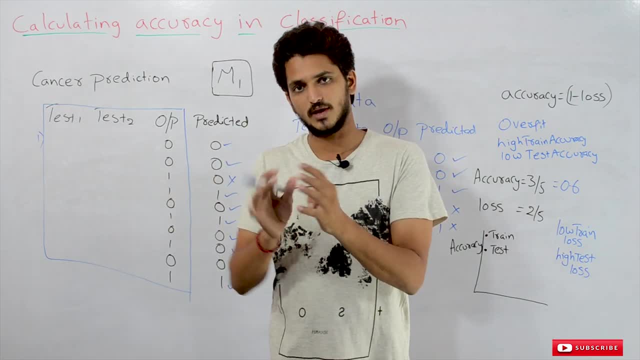 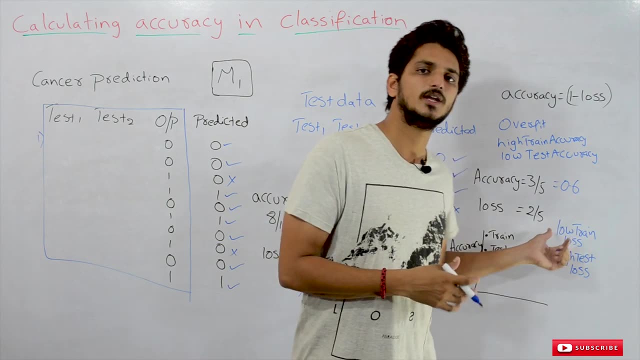 And we will find the best fit, also Where our model is going to fit the data correctly. So it is very, very useful in our models. Hope you understand the concept. If you have any questions in the concept, please post your questions in the comment section below. 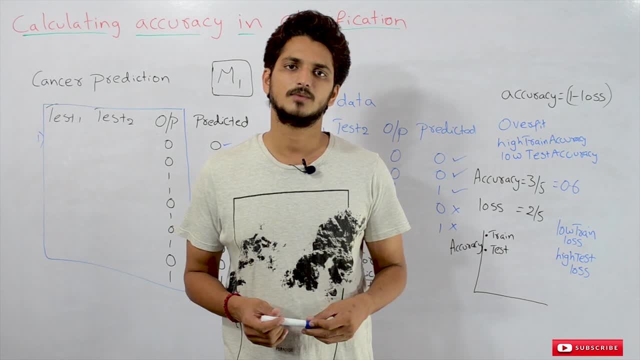 Thanks for watching. If you haven't subscribed to our channel, please subscribe to our channel and press bell icon for the latest updates. Thank you.